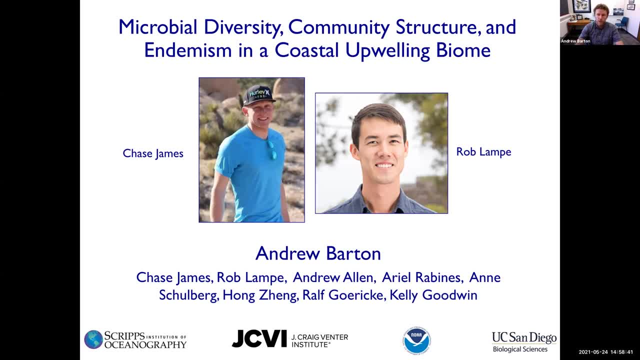 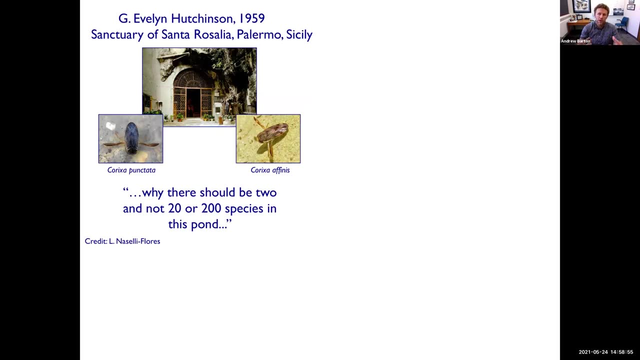 These are two up-and-coming students who I'm sure everybody will be hearing more of in the coming years. In fact, Chase James will have an e-poster which I encourage you to take a close look at. This session is talking about combining chemical, oceanographic and genomic measurements. 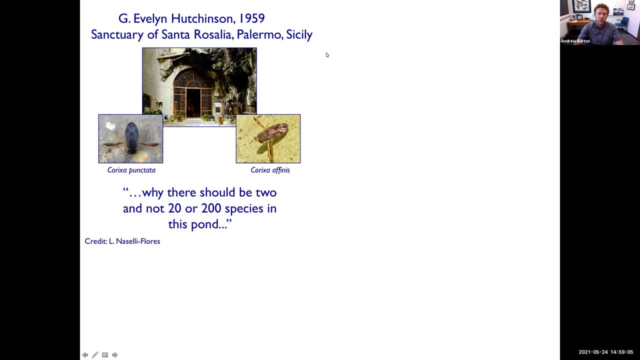 In so doing, there's the potential to answer many kinds of ecological questions. Evelyn Hutchinson famously visited this sanctuary of Santa Rosalia in Sicily. In a little pool near to the sanctuary There were two kinds of water, both coryxa punctata and coryxa finis. 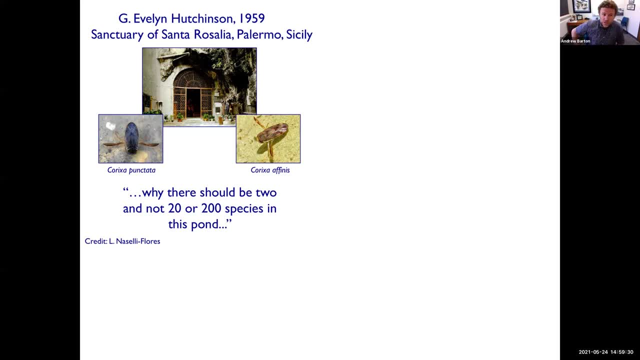 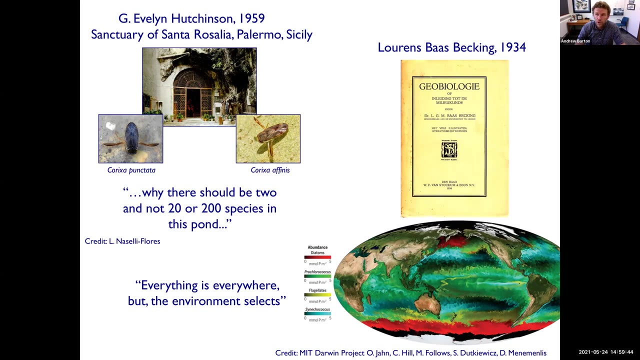 Hutchinson noted why there should be two or not 20, or 200 species in this pond. So ecologists have long wondered about the controls of biodiversity. There's also the Boss-Becking Hypothesis, which many of us have probably heard about. 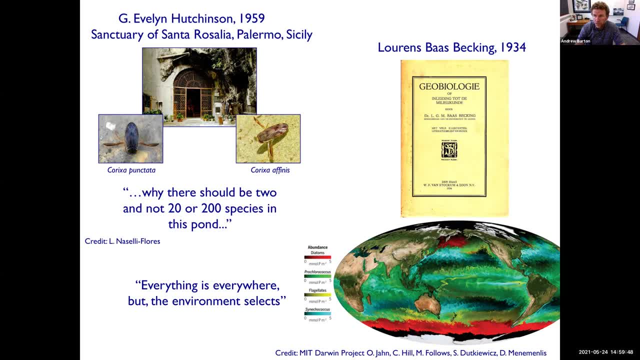 It basically postulates that everything is everywhere, but the environment selects. This is illustrated in the book, It's illustrated in this beautiful model simulation by the Darwin group at MIT, including Mick Follows, Stephanie Dukiewicz and collaborators, And here you see a global model which the different colors show you the kind of 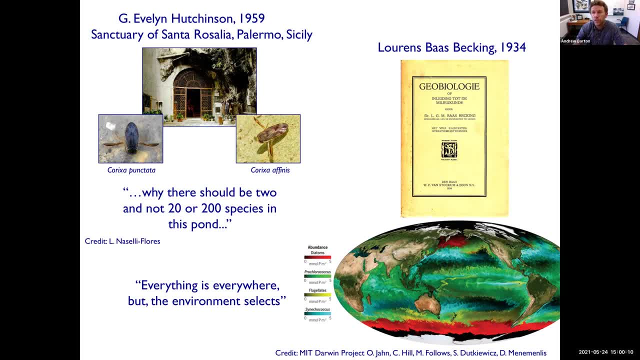 the relative dominance of different kinds of microbes living in different parts of the oceans, And so the basic idea is that the dispersal and population sizes of these microbes allow them to live everywhere, but the environment sort of picks who can live where And what relative abundance is. 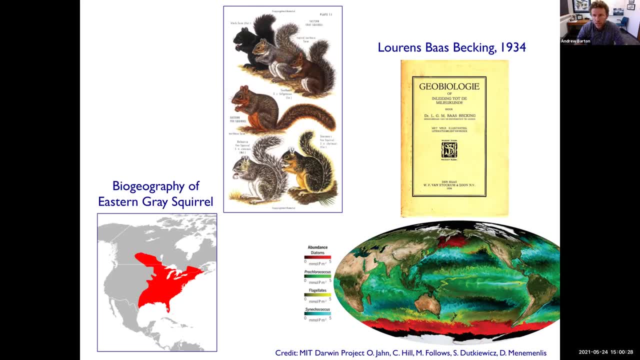 There's also this idea that you know we have a pretty good idea of where common organisms live, So you know. here's a picture taken from a mammal guidebook of different kinds of squirrels, And so I picked the eastern gray squirrel, which has this range, you see in the bottom. 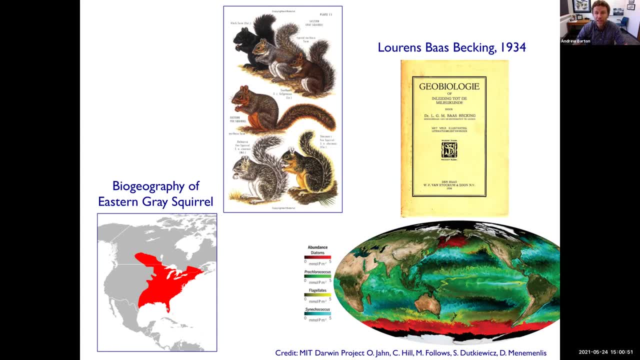 That's relatively well known, You know, you can go out, you can see it, And I would submit that nothing really similar exists for marine microbes, But that by combining all these different observations, perhaps ultimately we will know a map like this for the distribution of many of these marine microbes. 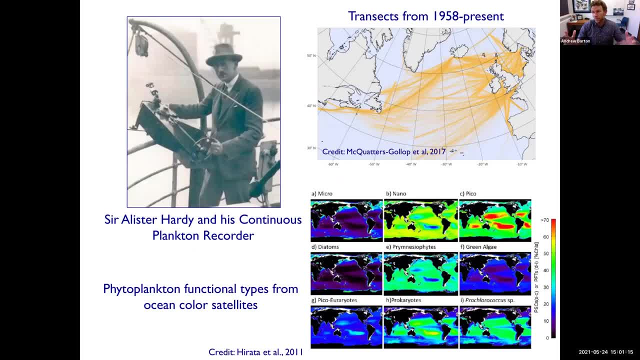 Now this is. I'm not saying that there haven't been a great deal of progress towards these goals in the last many decades, And there's some amazing examples. So Sir Alastair Hardy here has his famous plankton recorder And it was a very crude but effective instrument for sampling plankton in the ocean. 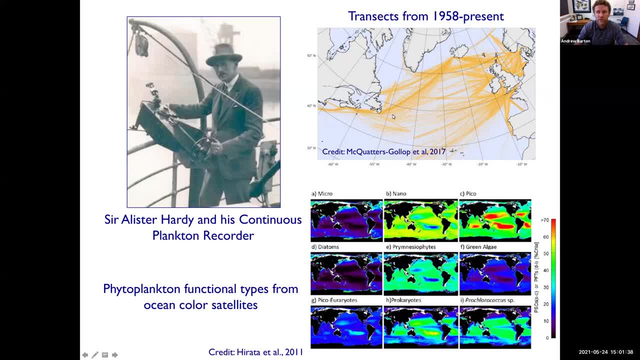 And it's towed behind ships. And if you see the tracks on the top right, if you are able to sample plankton across many places in a long enough time, you see how they change and how the biogeography of a lot of these organisms changes. 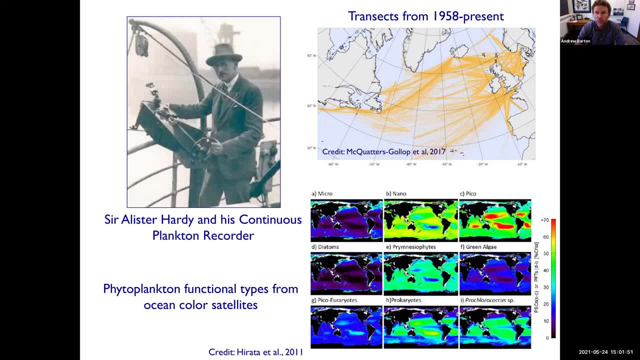 It's a spectacular resource for all of oceanography. And then there are satellite algorithms for estimating plankton functional types from space. Let me just show you here, Hirata 2011,. and you have, you know the different colors. show you. 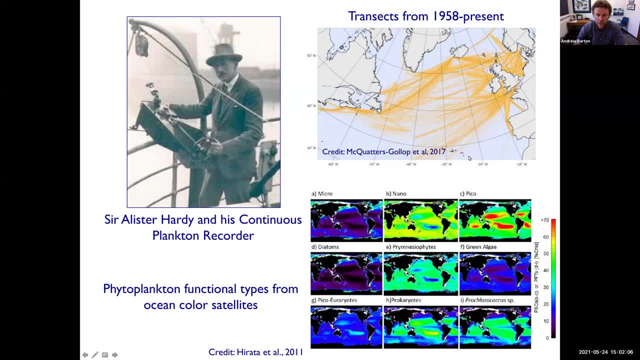 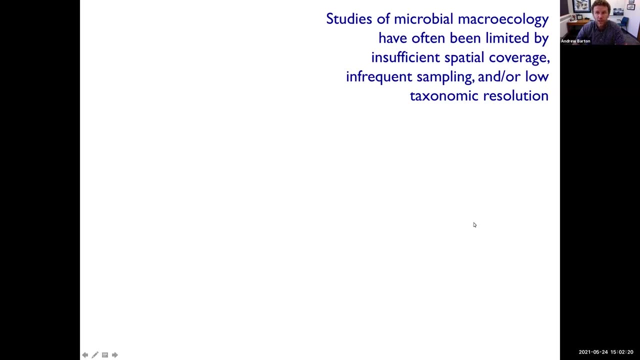 you know, the relative abundance of different kinds of plankton or phytoplankton. Here the colors are the percent of total chlorophyll. All of this is fantastic, But many of these you know there's a lot of research going on. 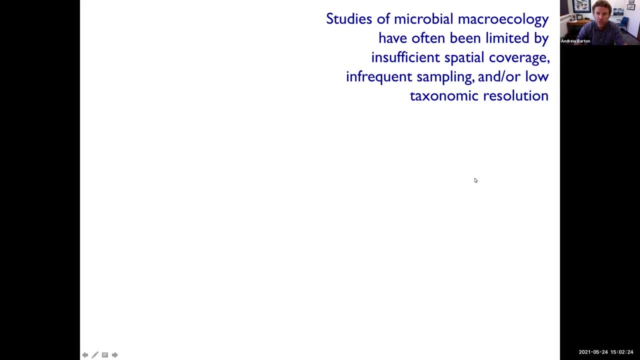 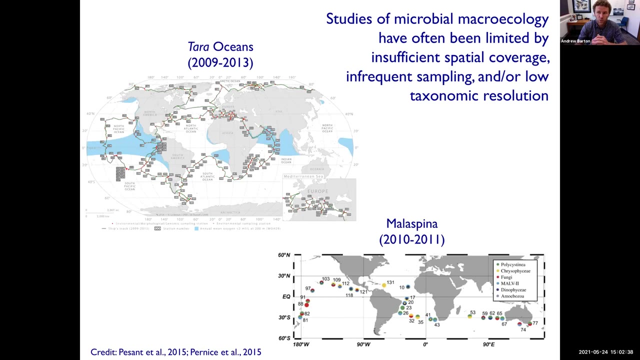 Many of these studies of marine macroecology have been limited by insufficient spatial coverage, infrequent sampling and or low taxonomic resolution. That's not to say not a great deal has been learned And that the doors have really been blown off in the last decade or so by these mega. 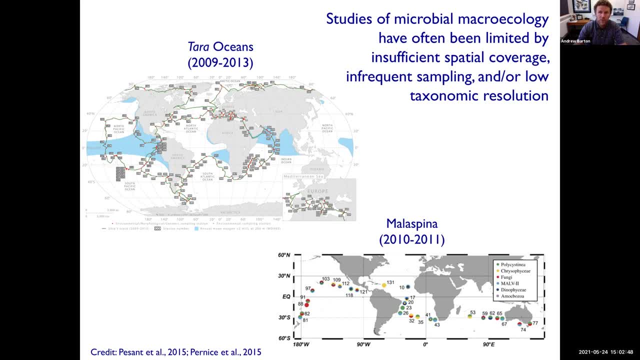 transect studies like Tara and like Molluscaena. The top left map Here shows you the distribution of Tara oceans samples between 2009 to 2013.. All and all major ocean gyres, Fantastic resource, Tremendous coverage across ocean biomes. 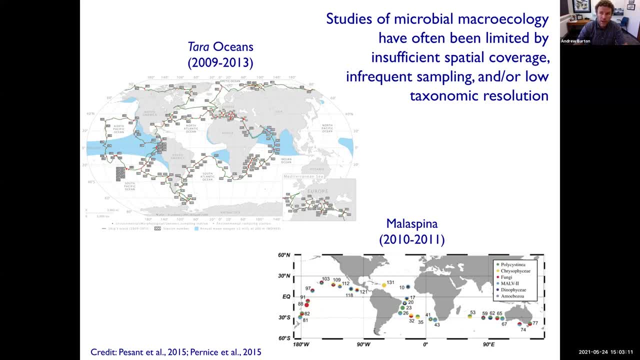 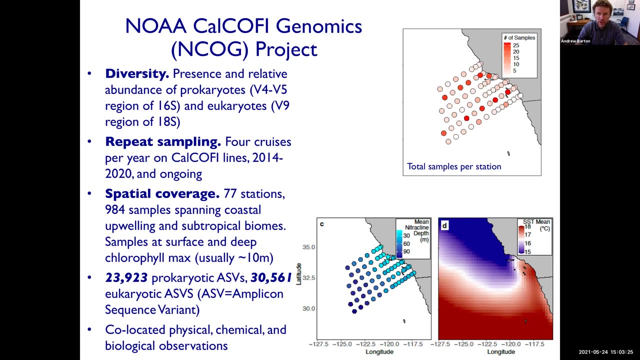 And something similar for Molluscaena, And a massive amount is being learned by looking at the. you know biodiversity of microbes from these studies, And what I really want to talk about today is another study in this vein called the NOAA CalCOFI Genomics or NCOG project. 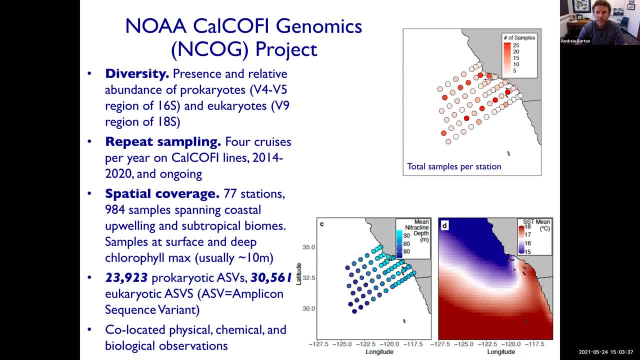 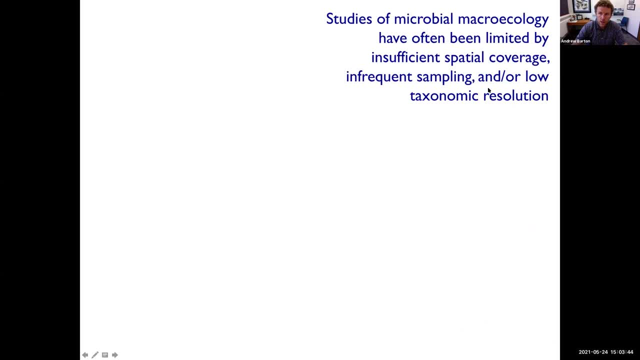 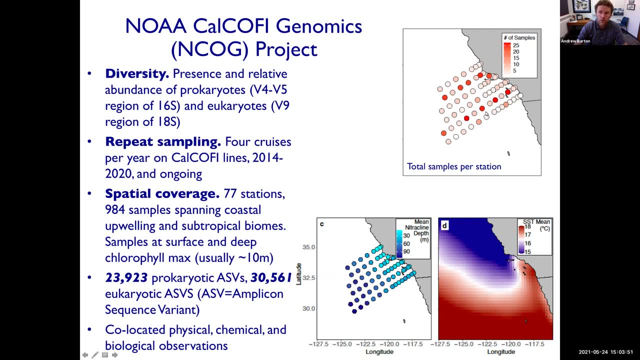 Now this is a survey along CalCOFI lines in the California current. You can see the data coverage here in the top right. This is the California coast Oops And the. you can see the different lines coming Sort of across from the coast. 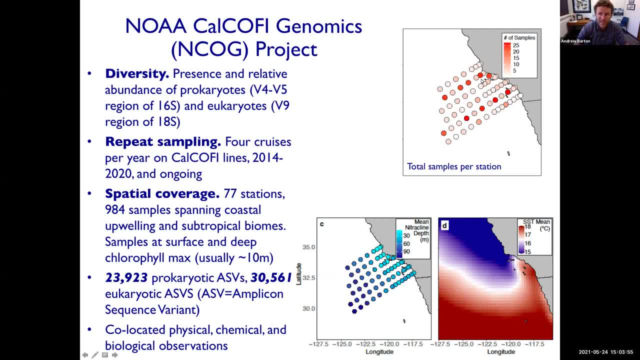 And then the colors. here are the number of samples that have been taken, And so this data set is incredibly rich. It was started by Andrew Allen and his collaborators in the lab, And it measures the diversity of prokaryotes and eukaryotes. 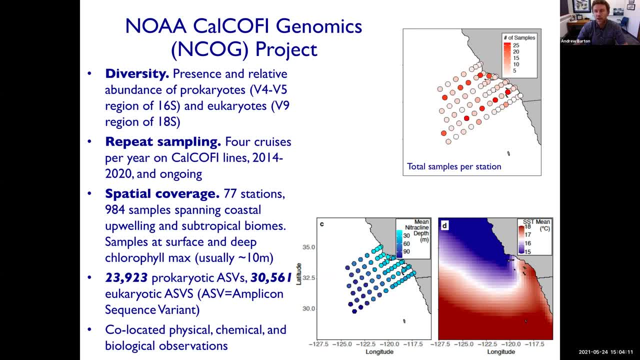 And so this is using the V4 and V5 region of 16S for prokaryotes and the V9 region of 18S for eukaryotes. Now what is interesting and unique about This survey is the repeat sampling. 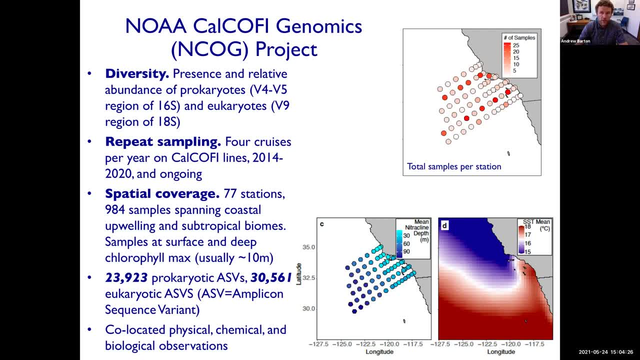 So there are four cruises per year on the CalCOFI lines, And this is the data I'll show you today, from 2014 to 2020.. But it is ongoing, You know, of course, subject to the funding, And there's this great spatial coverage. 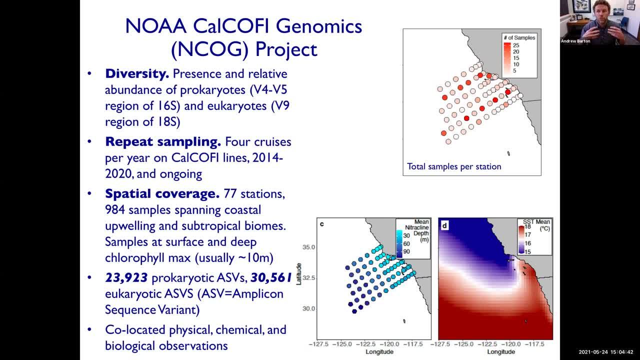 So you span from the coast in these upwelling areas to the subtropical biome offshore. So there have been nearly a thousand different independent samples taken And from that something like 50,000 distinct ASVs have been observed, Or ASV stands for amplicon sequence variant. 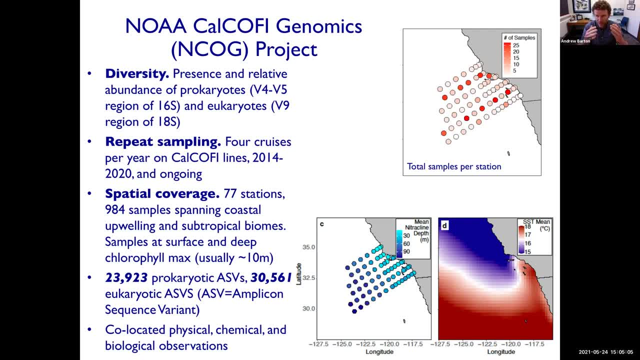 And that basically means they have an identical sequence to one another. What's great is that this survey- also because it's on the CalCOFI program or co-located with CalCOFI- also has co-located physical, chemical and biological. 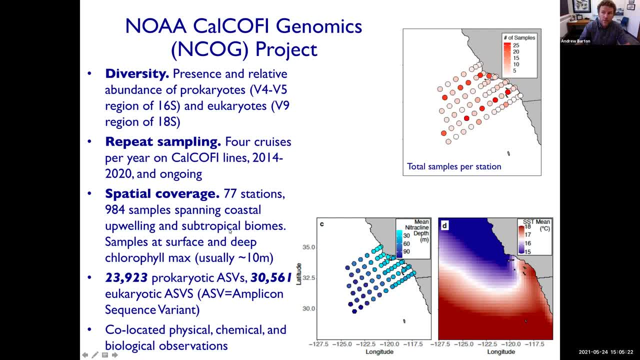 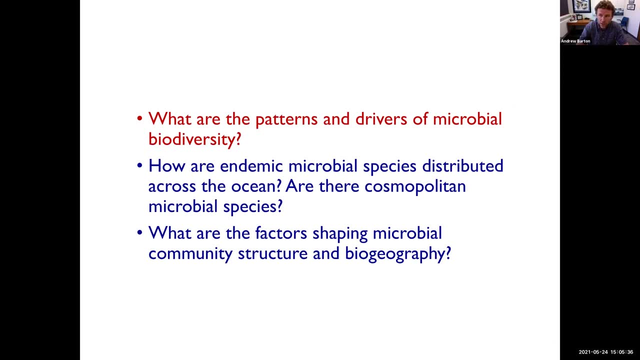 Observations. So this is a really unique resource that allows us to sample both time and space To learn about fundamental questions about microbial ecology in the ocean, And so I will just touch on a few today. These are obviously broad, I won't hit everything. 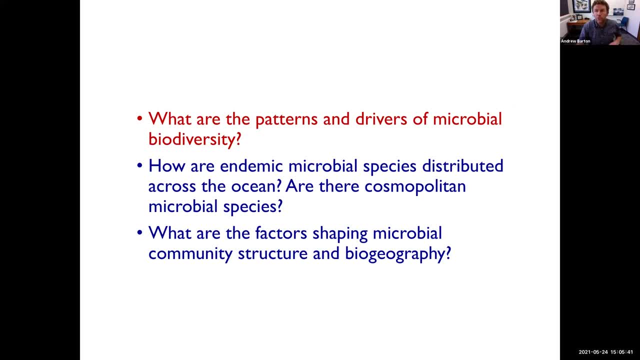 The first one I want to talk about is what is the patterns and drivers of microbial biodiversity, And then we'll talk about endemic and cosmopolitan species, And lastly, I'll just briefly hit On the factors that shape community structure and biogeography. 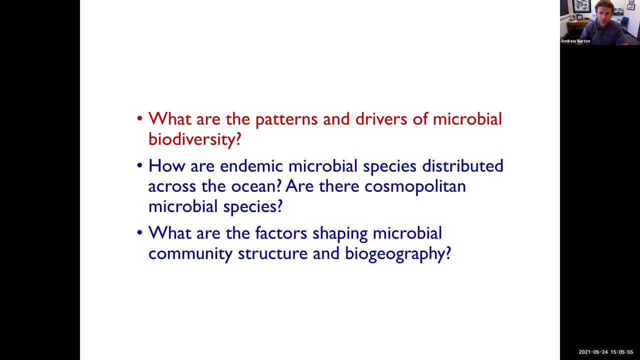 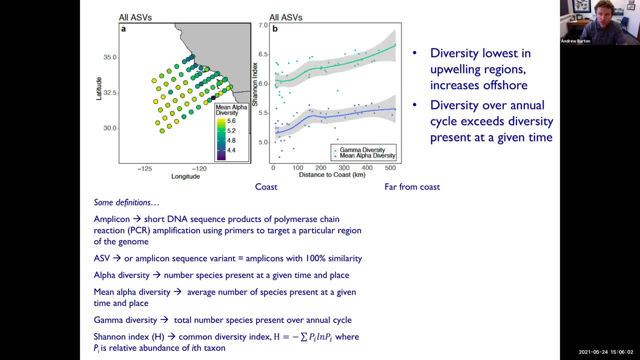 And I leave this topic mainly to Chase James's poster in the meeting. So what are the patterns of biodiversity in this region? So the unit I'll focus on here are amplicon sequence variants, or ASVs. You can think of an ASV as sort of like a taxon, sort of species-like. 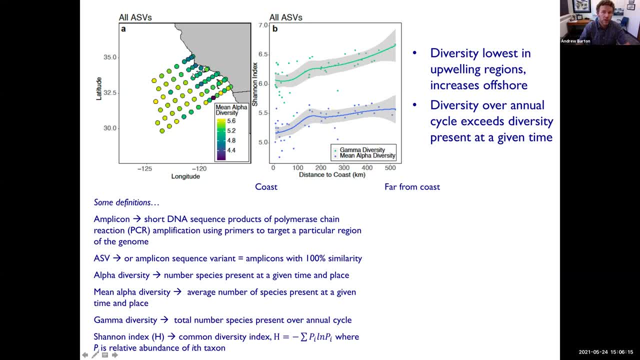 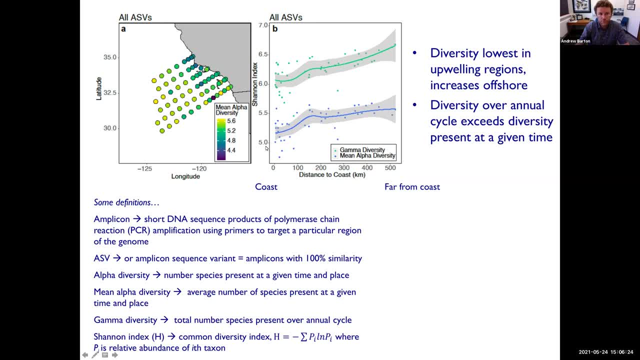 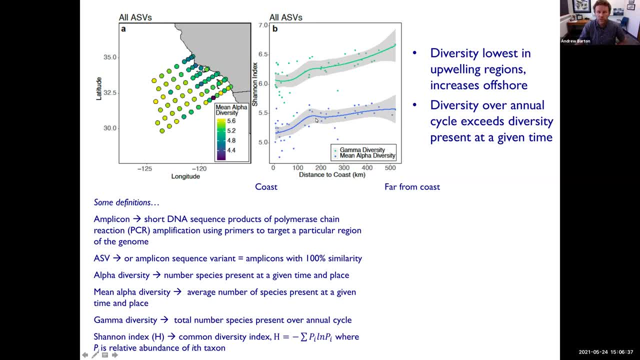 And the blue line is alpha diversity. Alpha diversity is just the average number or the number of species present at a given place and time, And so alpha diversity is lowest near the coast and it decreases away from the coast, And you can see that. 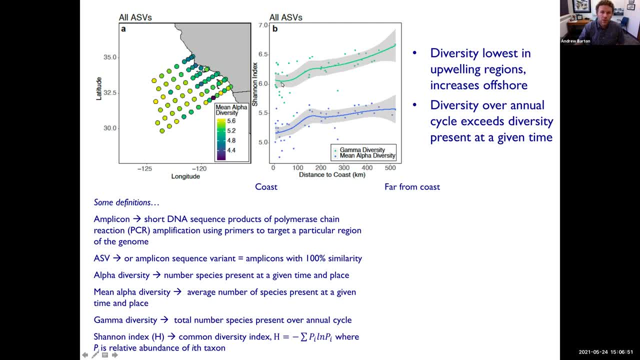 And now gamma diversity is just sort of this overturn, And here we define that as just how many species are present in total over the year. And so you see these two patterns, Basically higher diversity offshore, lower diversity near shore- And then when you look at the total species present over the year, it's higher than the. 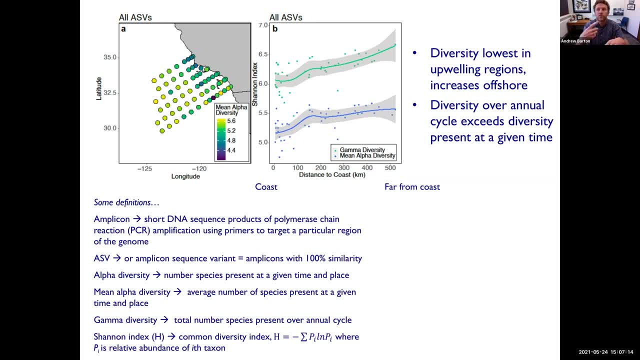 species present at a given time. That makes sense because you have this change in composition of the community over the time. The bottom left here is just various definitions. Given that you can stop and read those, I won't go through them, But that's just to make sure we have all the terms right. 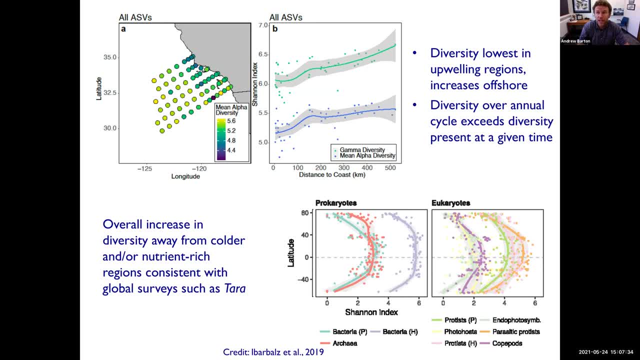 Now, does this pattern agree with what we found in other surveys like TARA? And the answer is basically yes. So this figure is from iBarBalls or eBarBalls- I'm not sure how you pronounce it exactly. Fantastic paper. 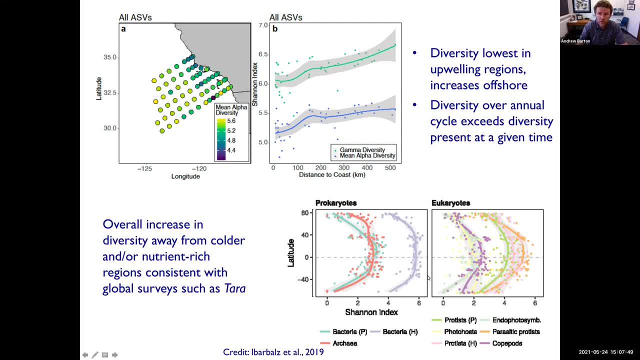 It summarized the soil. It's sort of latitudinal diversity gradients from the TARA Ocean's data, And we have prokaryotes on the left here and then eukaryotes on the right. It shows essentially that diversity is highest in the low latitudes and it decreases away. from the equator. This is similar in spirit to what we're finding here in this outflowing zone, That the more nutrient-rich and colder areas tend to have overall lower diversity than the warmer subtropical regions. So this is not to say that all organisms behave this way. 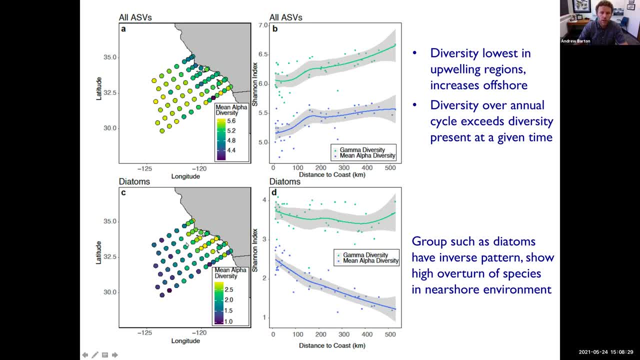 So, for example, diatoms show an inverse pattern. This figure on the bottom is just. the map on the left shows the mean alpha diversity for diatoms and it's highest near the coast And you can see that in this figure on the right. it summarizes that there's this opposite. 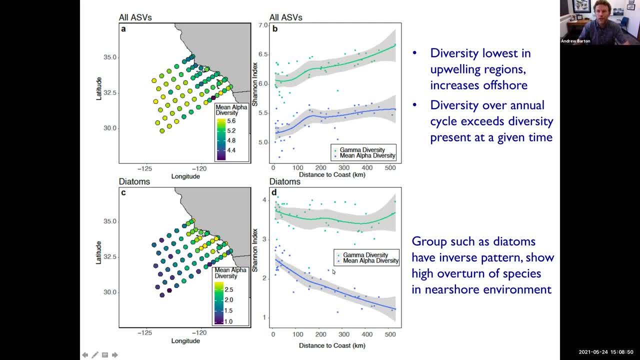 pattern from the rest right sort of the total microbial diversity. And so basically, what you find is that the diatoms you know slightly behave differently than other groups, And there are other groups that have that as well, And so I just want to stress that here. 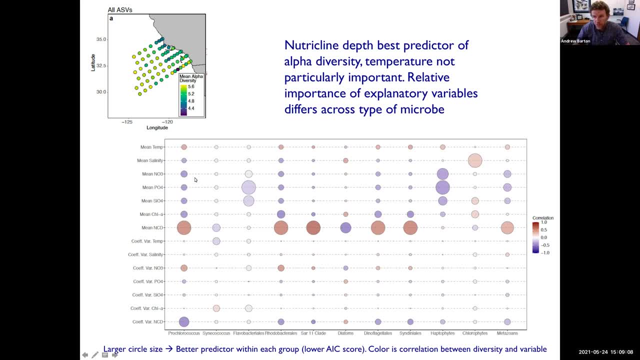 This is a lot of information here, but let me just explain basically what this means. So if you look on the Y, on the Y, you see all these different possible environmental factors that may influence the diversity pattern for different groups of microbes along the X axis. 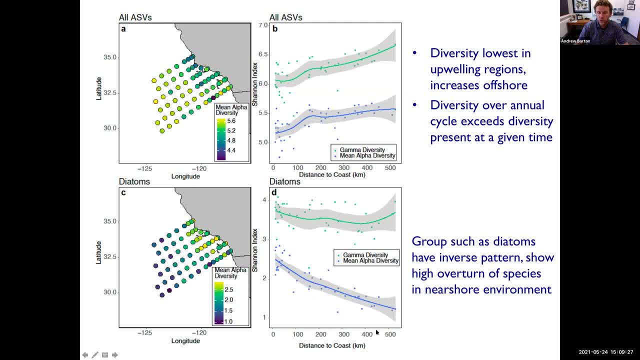 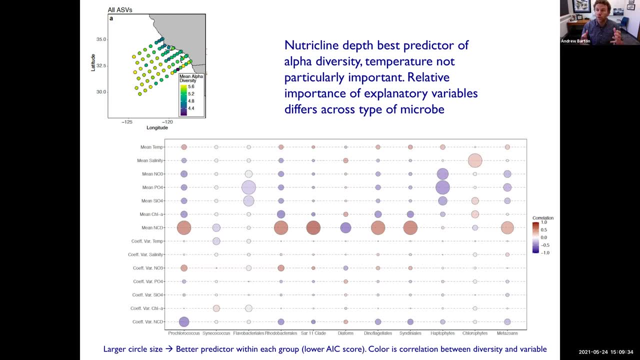 So Prochlorococcus, Sinicococcus, diatoms and so forth. The circle size tells you whether it's really important or not for that microbe. If it's important, it's big. If it's less important, it's small. 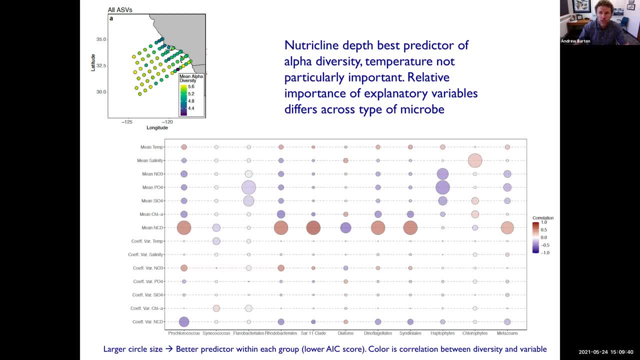 And that's determined by the AIC score from the GLM model. The color tells you whether that environmental factor is core or not, And so that's what we're looking at here. It's correlated, positively or negatively, And so the big takeaway here is a couple. 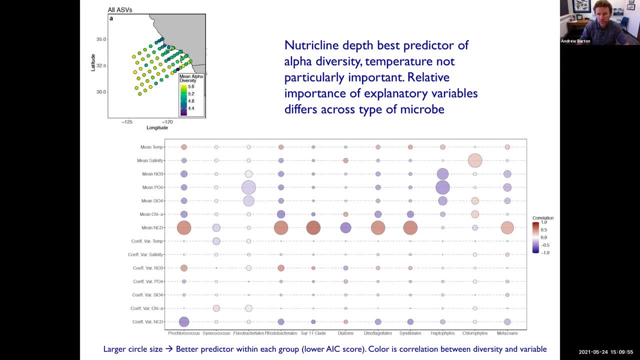 Number one. not all the groups have the exact same predictors. So you'll often see discussions in papers about well, what controls biodiversity, And the takeaway for me is that different groups have different factors controlling their patterns of diversity. But one can generalize and say that in this particular region, the provision of nutrients 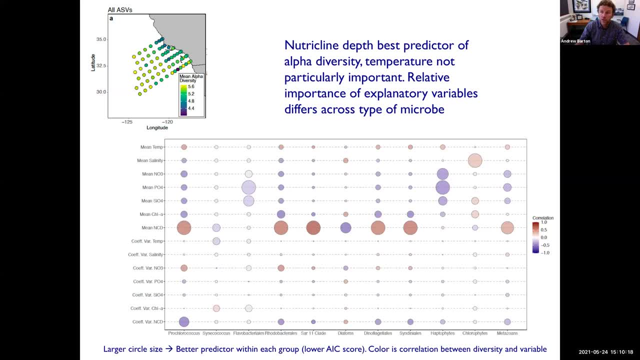 is very important in determining alpha diversity, Whereas temperature, which is often speculated to be a really important factor, does not really appear to be that important here, And you can see that if you look across the rows mean temperature, you look across these. 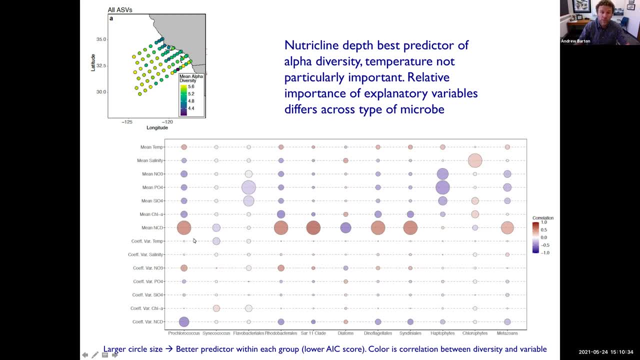 rows: yes, it's not negligible, but it's not nearly as important as nutrient supply And in this context, nutrient supply. for that we're using a proxy which is the Nutri-Client Depth or NCD. So it's not negligible, but it's not negligible. but it's not negligible, but it's not negligible. 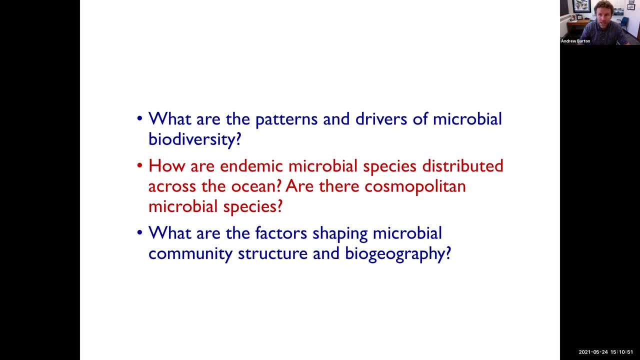 Next, I want to talk a little bit about endemic microbial species and how they're distributed across the ocean, and also cosmopolitan microbial species, And I hope you'll see how this connects with that. everything is everywhere, theme that I brought up in the beginning. 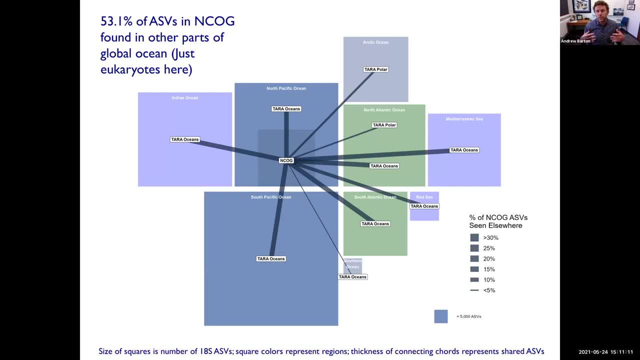 So just to sort of step back and place some of these data in context, this is a really interesting figure. This shows you essentially how the ASVs in the NCOG survey in the California Current are linked to other areas of the ocean from TARA. 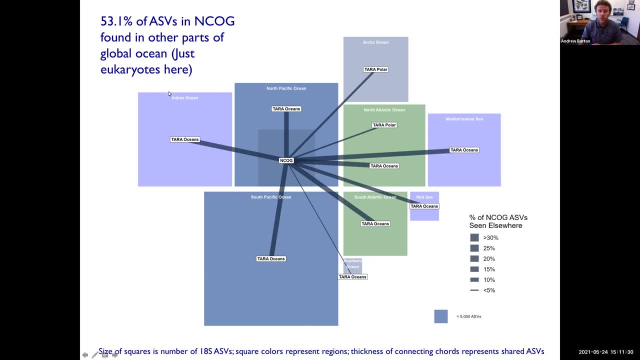 So each box is a different region of the ocean and the size of the box is the number of ASVs or amplicon sequence variants that are present. This figure is just for 18Nets for eukaryotes. 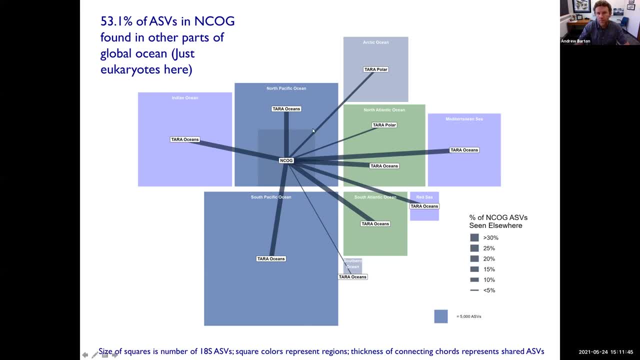 And here in the middle you can see the NCOG, And so just looking at it closely you can see. okay, the number of species, or ASVs, in the NCOG area is less than the whole North Pacific Ocean. 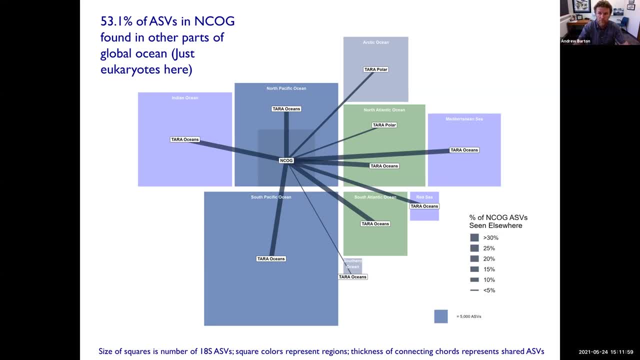 That makes sense because you know the North Pacific Ocean is bigger. The bars here show the degree of similarity with other regions of the ocean. So basically, how many of the ASVs in NCOG are found in the South Pacific Ocean North? 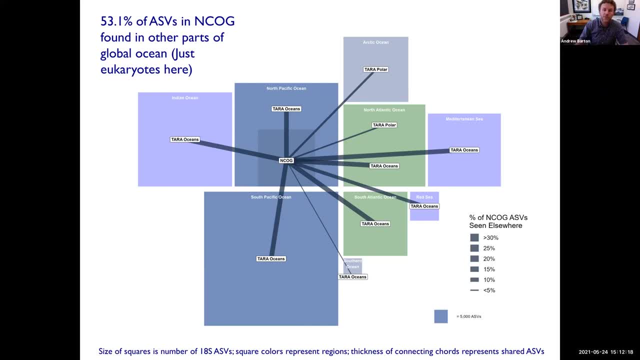 Pacific Ocean et cetera. So it makes sense. There's not a lot of overlap with the ASVs in the Southern Ocean or the Arctic, but there's quite a lot of overlap with nearby regions And generally the overlap decreases with distance. 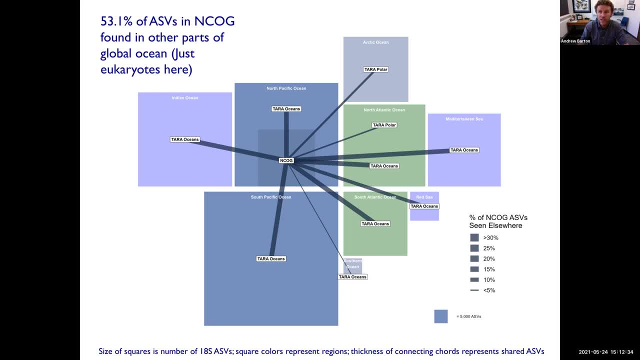 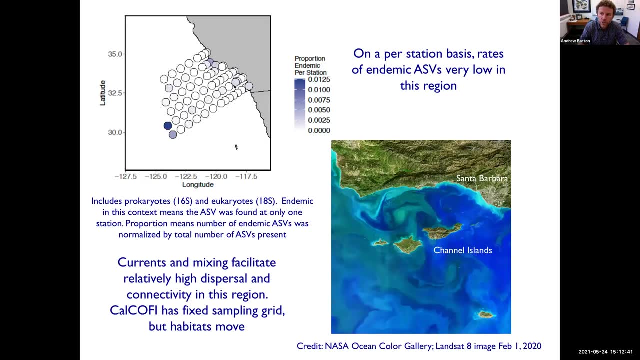 So, overall, something like 50% of the ASVs in the NCOG project are found somewhere else in the global ocean than TARA, And so we took this to basically ask you know, are there any indemnifications? Are there any endemic species in this region, the NCOG region? 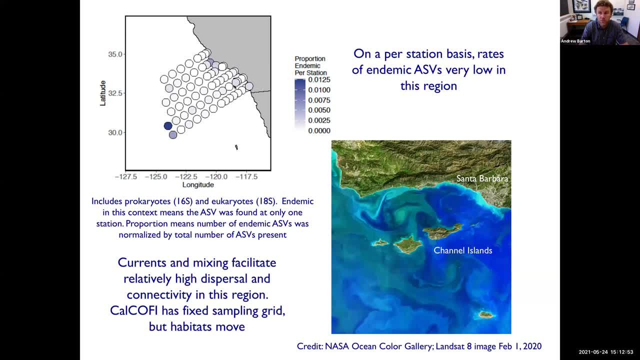 So we essentially calculated, on a per station basis, the rates of endemism, And so for each NCOG station we asked: are there any ASVs that are found only here, at this one station? Maybe, not surprisingly, very, very few of the ASVs are, you know, endemic to one station. 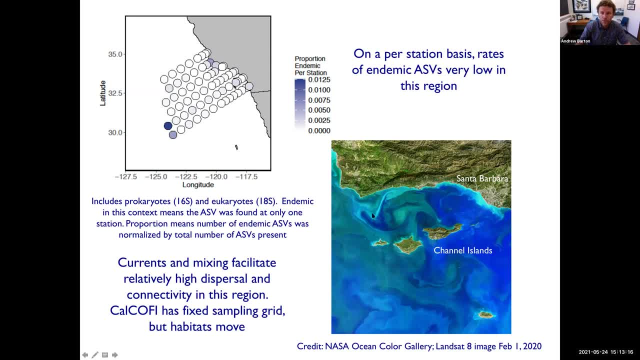 So that may seem obvious if you look at this picture in the bottom right here. This is a Landsat image showing mesoscale and submesoscale features in the ocean. This is, you see, the plankton, phytoplankton, chlorophyll. 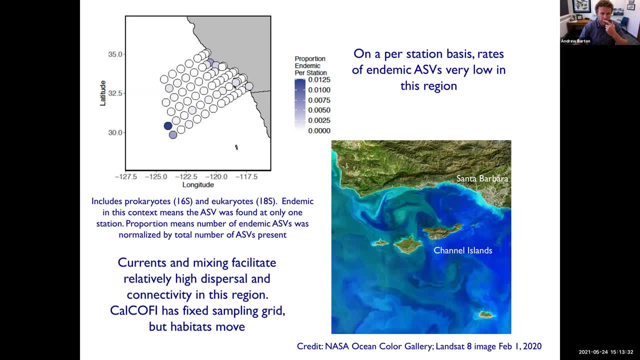 You also see all the fronts, filaments. There's a lot of currents and a lot of mixing that facilitate high dispersal and connectivity throughout this region. So you know there's a great amount of exchange between these stations. The potential for them to have truly endemic species is quite low. 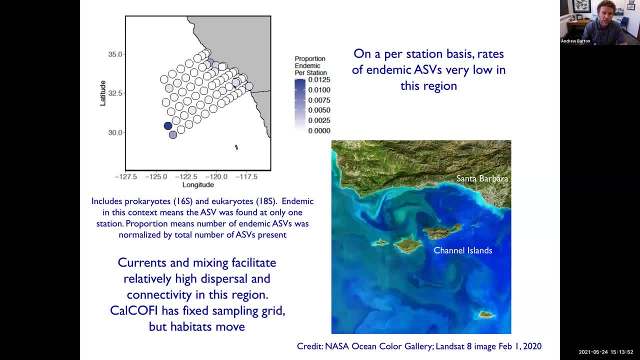 But leading into the next slide, really. so this cow coffee grid is fixed sampling, But these habitats, you know, offshore, nearshore, they move around, And so what we sought to do was to be able to basically quantify where the habitats were. 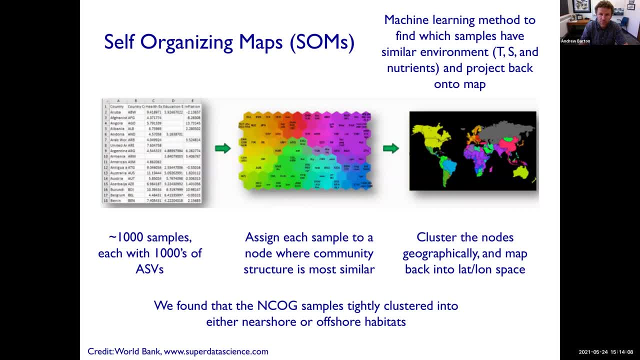 and then ask whether the habitats have endemic species. To do this we use a machine learning tool called self-organization. It's called self-organizing maps. Basically, the idea here is you're finding which samples have similar environments And you're going to project that back on the map. 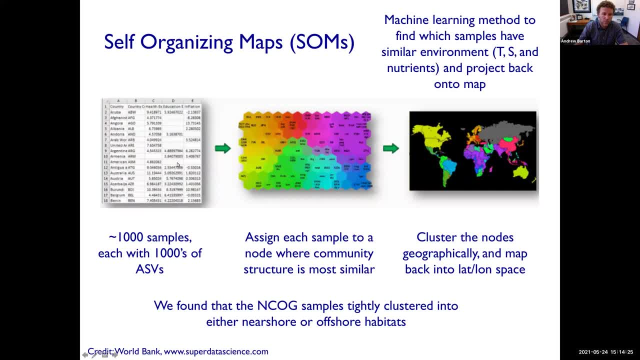 So a classic, famous example is for basically all the countries on Earth and all these metrics of human health and well-being, And then you cluster all of the different countries based on these metrics into different nodes And this map here in the middle, each tile: 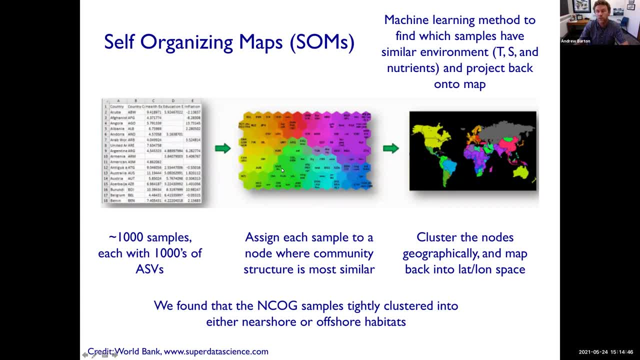 or so. each node here has countries that are most similar to each other in terms of human health and well-being, And then you can cluster them based upon similarity between these different nodes, And then you can project it back onto a map And you can basically find certain regions and 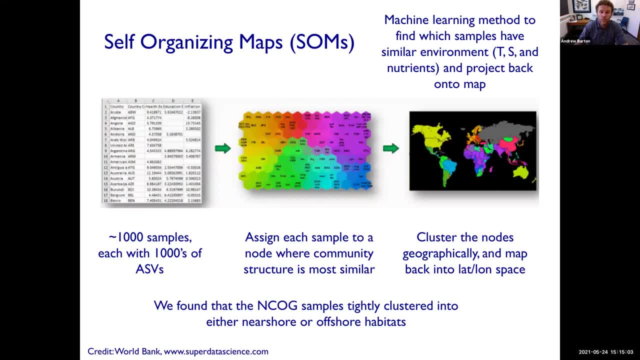 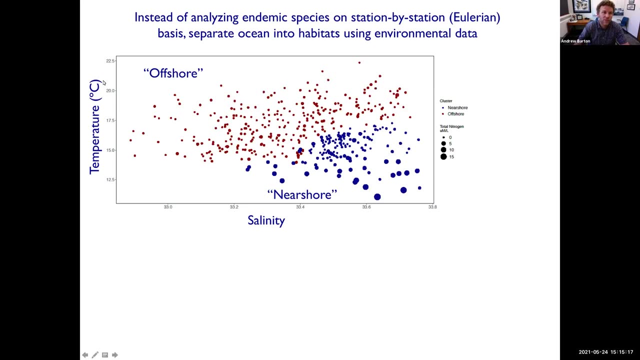 countries have similarities or differences on human health and well-being, And so we do something like this for the environmental variables, that are, temperature, salinity and nutrients, to try to separate out habitats. Just to illustrate how that works, here's temperature on the y-axis: salinity. 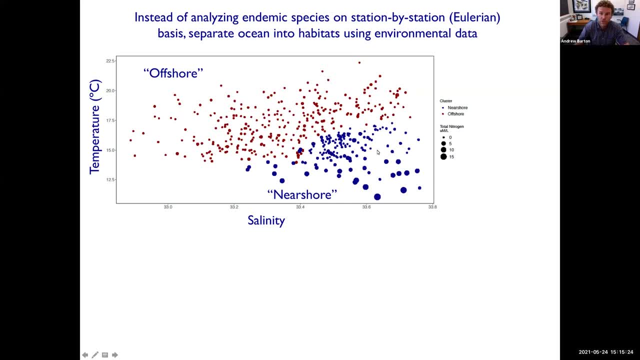 on the x-axis, and then the size of the circle here is total nutrient, And so the red dots are the sort of offshore cluster and the near-shore cluster are the blue dots, And then we found basically the number of the ASVs that were endemic to that habitat, Rather than this Eulerian stance. 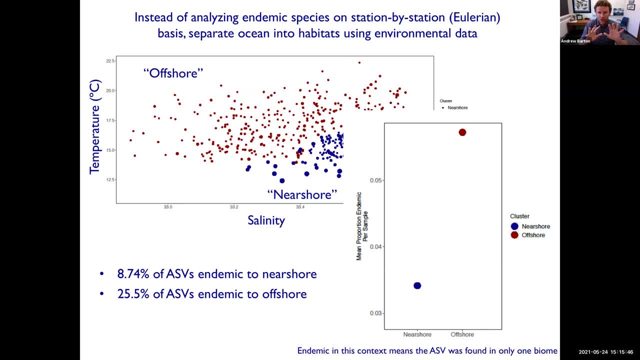 you know this, you know station by station basis. we said we know these habitats are moving around. Let's just calculate the number of endemics per habitat And when you do that that rate of endemism goes up And we find that about 8.74 percent of the ASVs are endemic to the near shore. 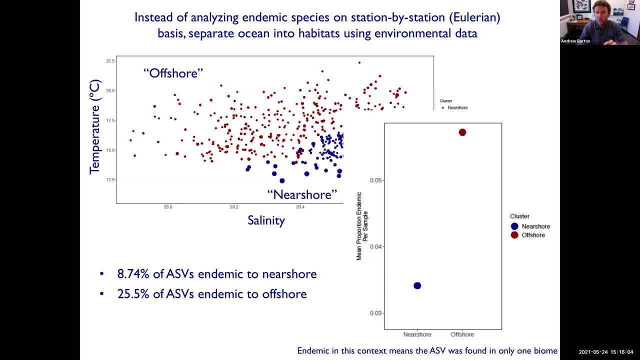 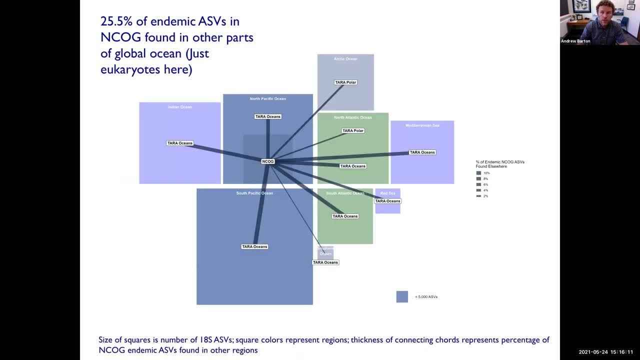 And then 25.5 percent are endemic to the offshore, So offshore endemism rate is notably higher. Now, that is not to say that some of those endemic species in this region aren't found somewhere else, And so, in fact, we compared this back to the Tara Oceans data and we found about 25 percent of those you know. 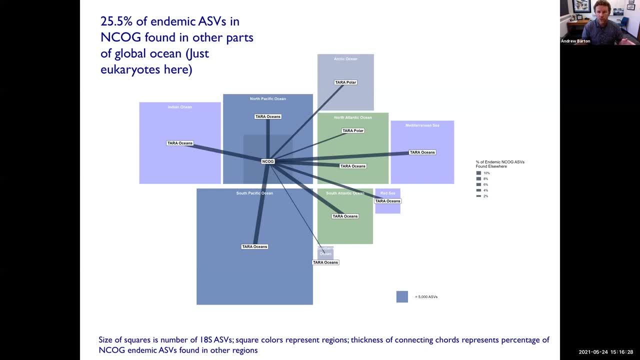 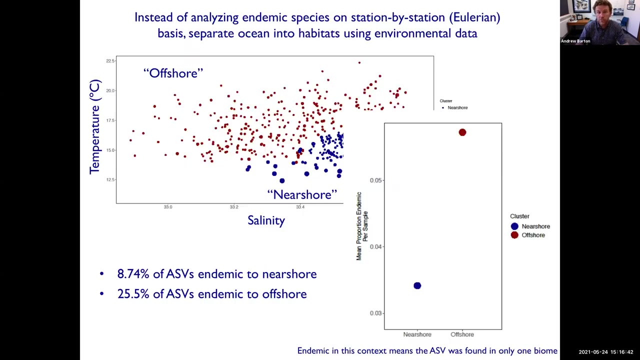 regional endemics from the ANCOG are found somewhere else on Earth, in Tara. So you know, some of those endemics are probably not found anywhere else on Earth but some of them are. But we hope and think that this, this pattern of this kind of near-shore offshore gradient is robust and it's a very interesting 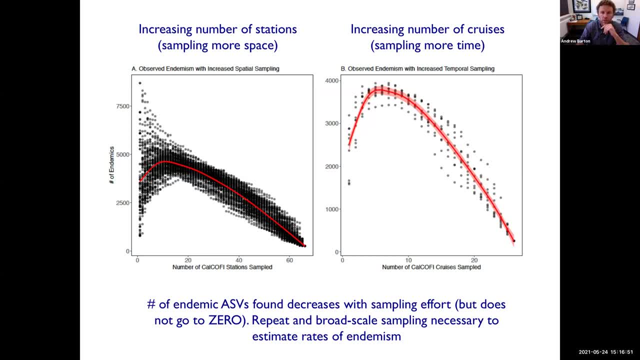 one. Another interesting, I think, takeaway for how to think about this is related to sampling effort. So two plots here: On the y-axis, in both is the number of endemics, and on the x-axis is basically the number of stations sampled on the left and on the right is the number of. 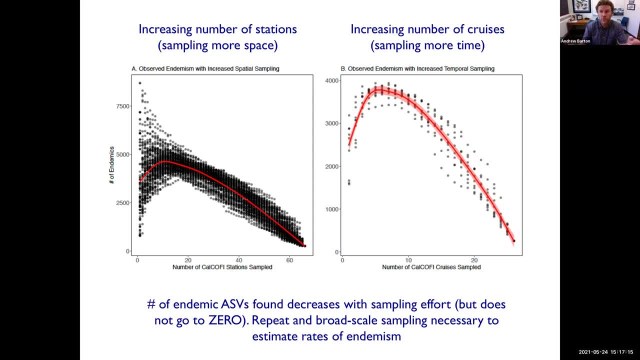 sources, And this is all for just the Noah Calcott Genomes Project data, And so the takeaway here is that the more you sample, you're likely to find fewer and fewer endemics, because you are really you know, you sample the heck out of it A lot of those things that you found. 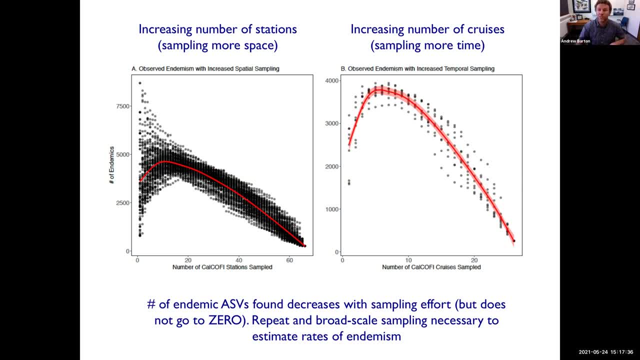 you know in just one spot. if you look long enough or hard enough, ultimately you're going to find it somewhere else. But the other thing here we found is that it doesn't go to zero. We We have no evidence that it goes to zero. 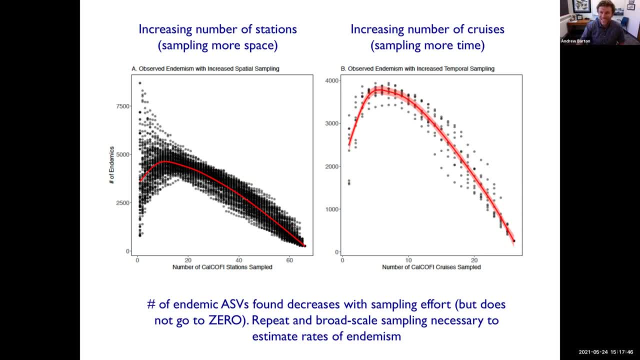 And so we do think there are things that are truly endemic to the Southern part of the California current ecosystem. But your ability to find them and your estimate of rates of endemism is gonna be critically tied to how frequently and broadly you sample. So we think that repeat and broad scale sampling 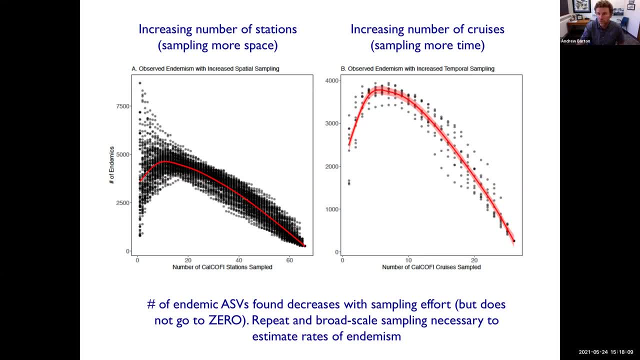 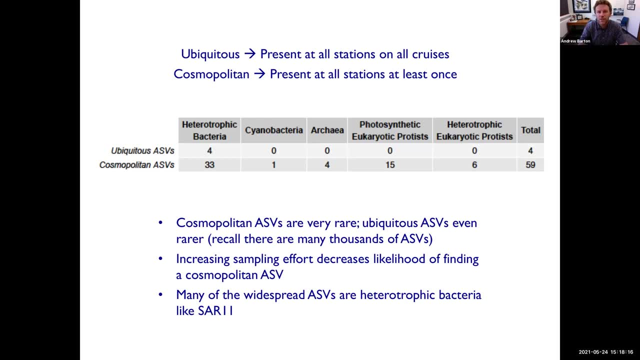 is really crucial to study patterns of endemism and biodiversity among marine microbes. Now, another interesting thing is this concept of cosmopolitanism. So if everything is everywhere, one might expect that in theory, you could find lots of microbes in virtually everywhere. 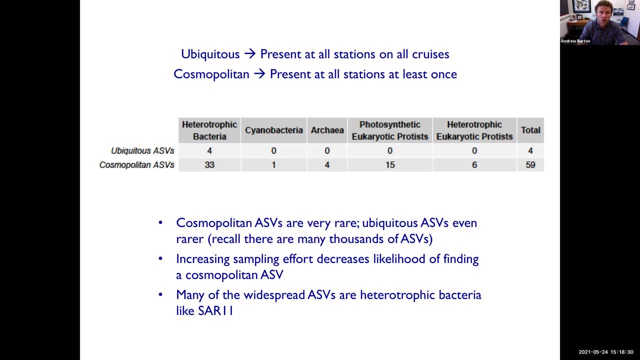 So we, using the data from NCOG, we looked for ubiquitous and cosmopolitan species. So we define ubiquitous species as something that's present at every station and every cruise, Which is obviously a high bar, And cosmopolitan is an organism that's found. 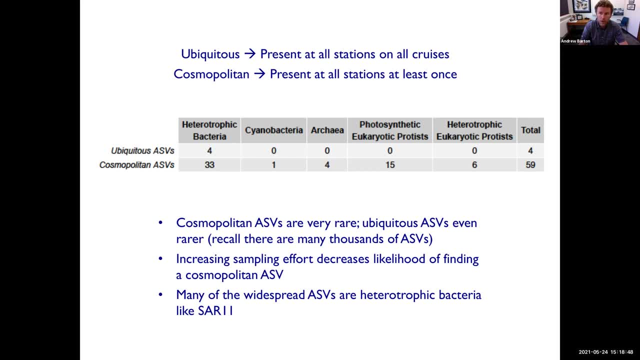 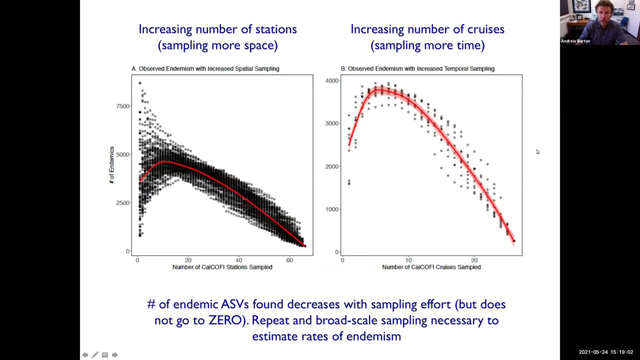 at every station at least one time, And this table here summarizes the total number of ubiquitous in the top row and total number of cosmopolitan in the bottom row- ASVs. And I just wanna point out these numbers are very, very low. So cosmopolitan ASVs in this region are extremely rare. 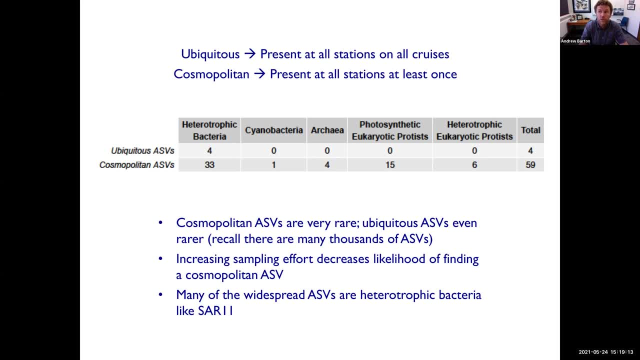 And ubiquitous ASVs are even rare. still Recall that the total number of ASVs is in the tens of thousands. So these are very, very small proportions. Like endemism, when you increase sampling effort it decreases the likelihood of finding a cosmopolitan ASV. 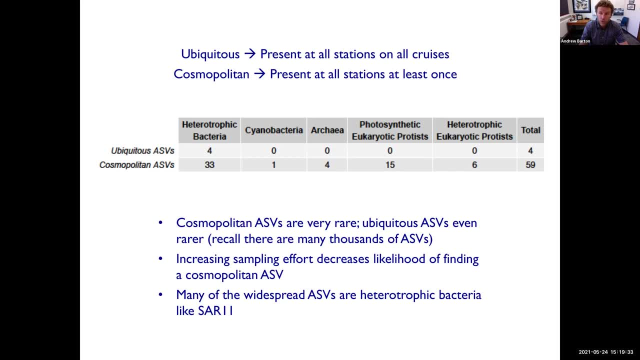 Interestingly, the organisms that are really widespread tend to be heterotrophic bacteria like SAR11.. That makes sense, and they have small size, great dispersal rates and huge populations. So, for example, these 33 of the cosmopolitan ASVs- many of them are different ASVs of SAR11.. 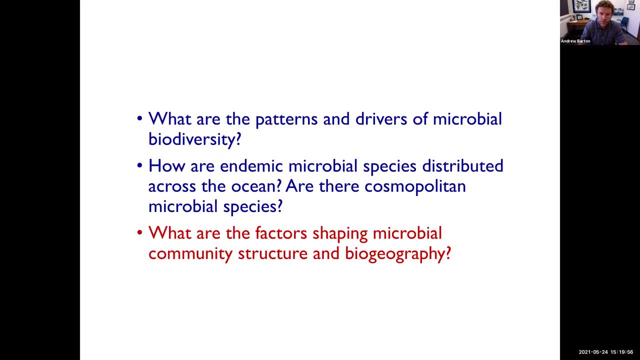 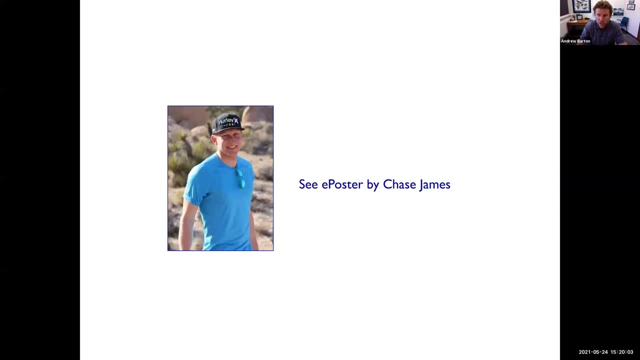 So last theme to talk about is: what are the factors shaping microbial community structure and biogeography? For this I refer you to a great e-poster by Chase James. Chase has been doing excellent work in understanding factors that really shape microbial communities, and all I will say as a teaser is that 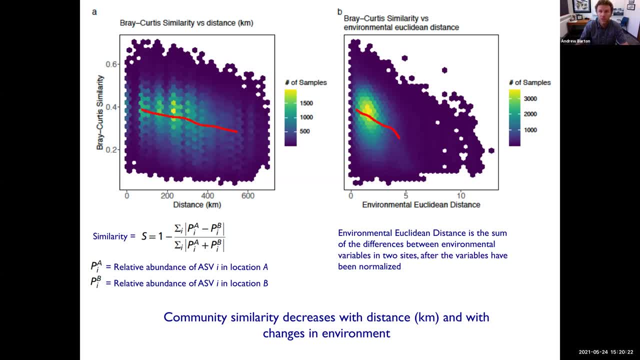 changes, environment structure, microbial communities, And so this plot on the left shows that Ray Curtis, community similarity versus distance, and then on the right is Ray Curtis, community similarity versus Euclidean environment. So So, essentially, how different is the environment? And so there's, you can see a steep decrease here and a more flat decrease in the lift. 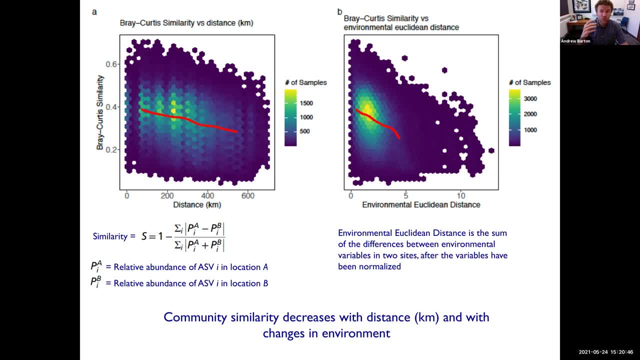 And that tells you that environmental change is a really strong factor shaping microbial community similarity. This is relevant because there's a lot of discussion about whether dispersal and neutral processes are important in shaping microbial communities or local environmental selection. See Chase's poster for more on this in more detail. 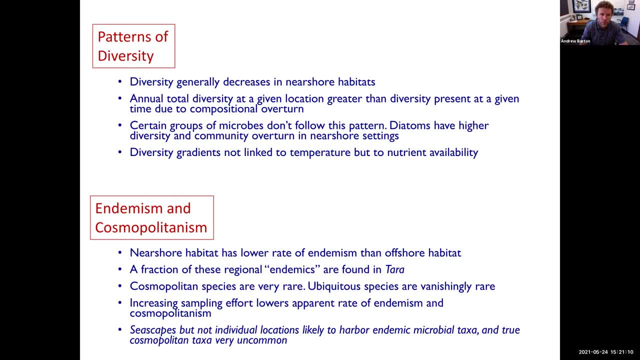 So some takeaways, just a- you know, brief overview In terms of pattern diversity. diversity generally decreases in near shore habitats. The annual total at a given location is greater than the diversity present at a given time due to this computational or compositional overturn. 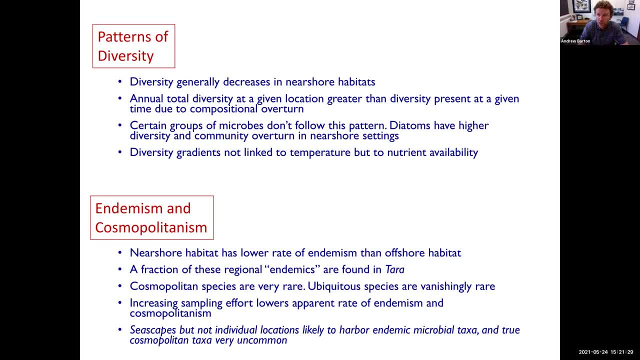 Certain micro groups don't follow this pattern. Diatoms are an exception. They have higher diversity near the shore And the diversity gradients do not appear linked to the temperature, or do not appear linked to temperature but to environmental or nutrient availability instead. So some of the global surveys suggest that temperature is really important. We're showing that in this region that's not the case. 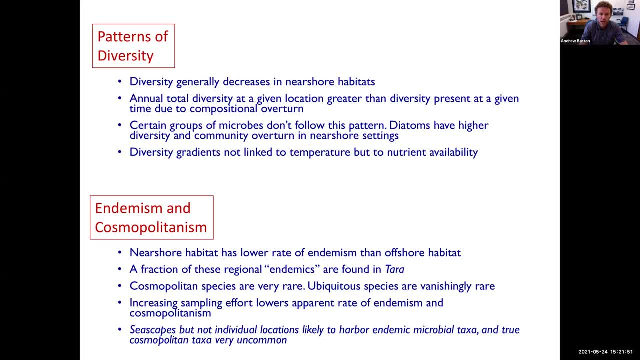 Now, in terms of endemism and cosmopolitanism, near shore habitat has a lower rate of endemism than the offshore. Now, many of these regional endemics are also found in Tara, But one thing that's clear is that the cosmopolitan species are extraordinarily rare and that the ubiquitous species are almost non-existent. 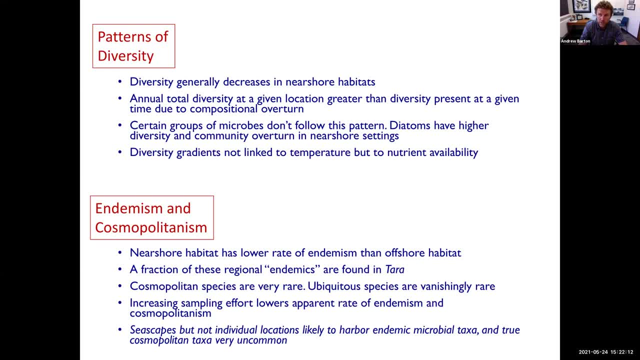 Sampling effort. obviously has an important influence on this- And this is an emerging picture- is that seascapes have endemic species but not necessarily invictable locations, So the appropriate unit for thinking about where endemics live in the ocean is like a habitat that is similar. 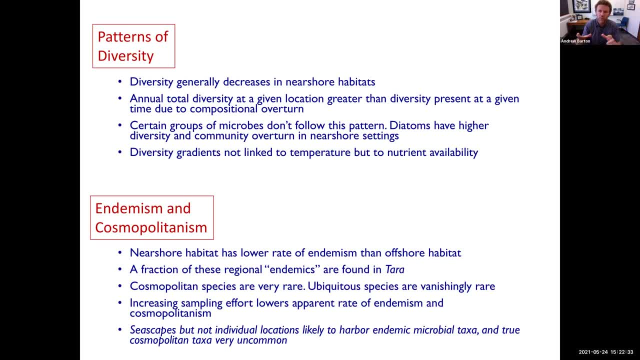 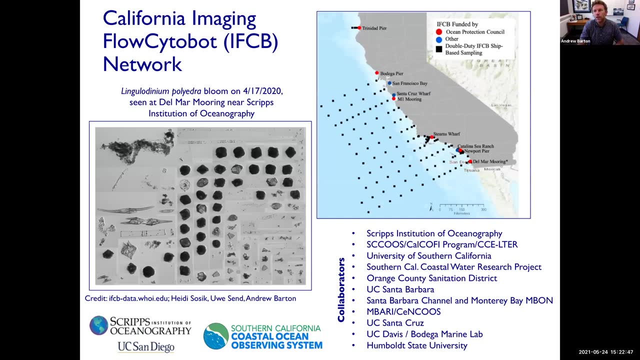 That's sort of like a biome or a habitat, but it moves around in time. So you have to track those moving habitats and look for the changes in community structure within them and then the endemics and diversity within them. Lastly, you know genomics are but one way of sampling the ocean. 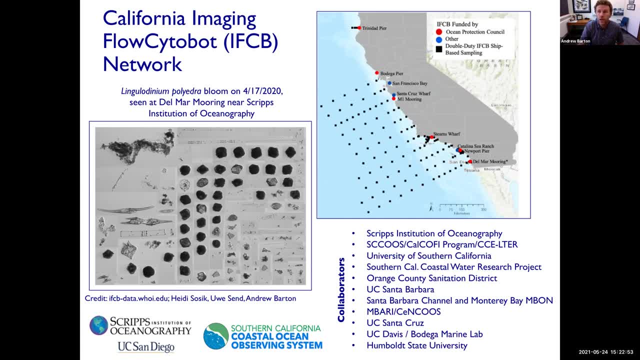 So I just wanted to highlight an additional tool that I and many others are working on, And this is the California Imaging Flow Cytobot Network. So basically, along the California coast, where there are these red circles, we have or are deploying soon, imaging flow cytobots. 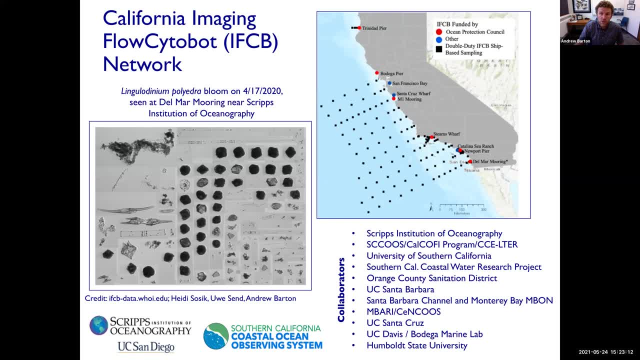 These take pictures of microbes in situ and you can use different tools to identify them to species level. So with this tool you'll be able to understand things like harmful algal blooms. also, compositional change through time: effects of regional and global climate change. 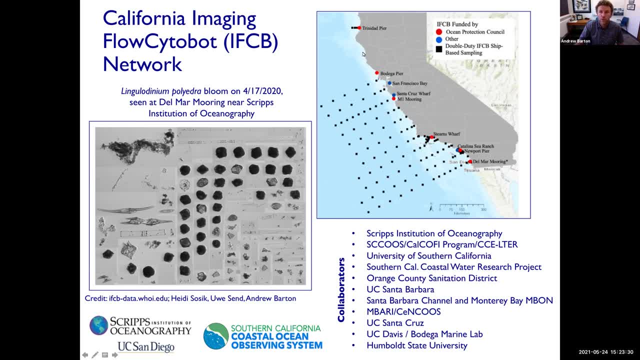 So this is going to be a great tool. It's a really powerful tool for analyzing how microbial communities along this coastline change. There's a huge network of collaborators involved here and this is hopefully a long-term project, But I believe that this linkage of genomics with these imaging tools is a really powerful way forward to thinking about both changes in community structure and diversity at the time and in space. 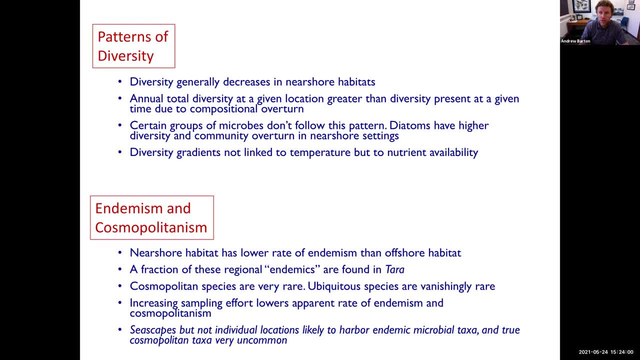 With that, I really want to thank you all for joining us. Thank you. I want to thank the organizers of the OCB workshop and also the organizers of this session in particular for inviting me. I look forward to a conversation during the actual day of the session. Thank you. 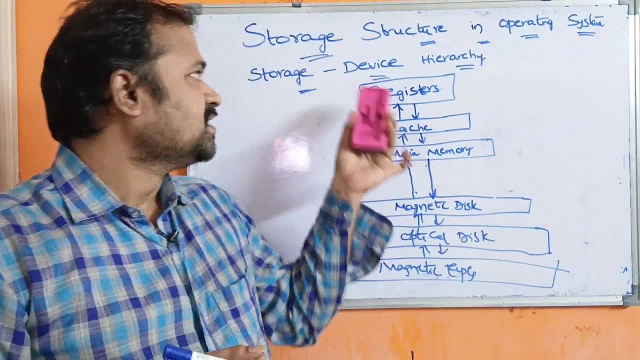 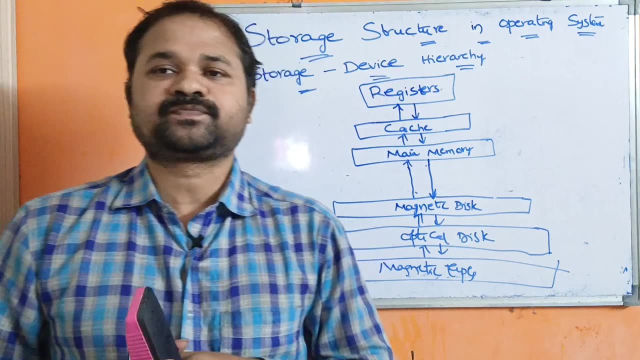 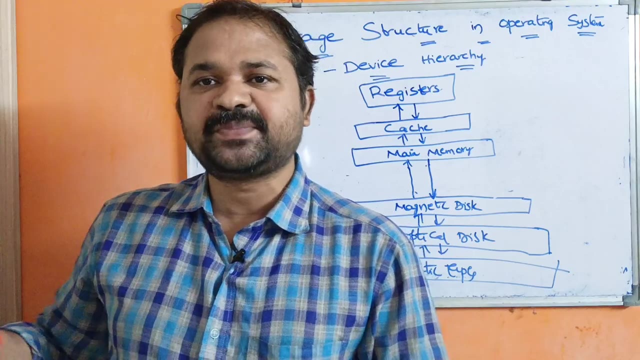 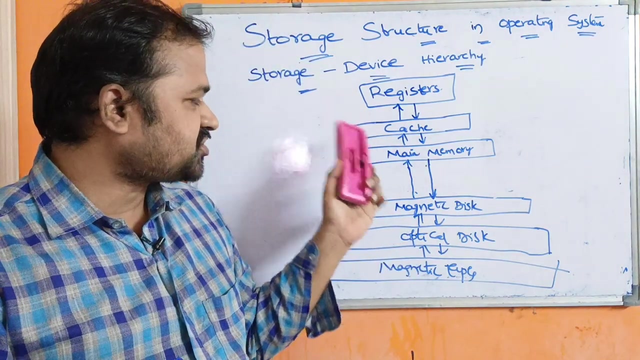 In this video we are going to discuss about storage structures in operating system. that is nothing but storage device hierarchy. Storage devices are mainly useful in order to store information in the computer. We have different types of storage devices, such as register, cache, main memory, magnetic disc, optical disc, magnetic tape. 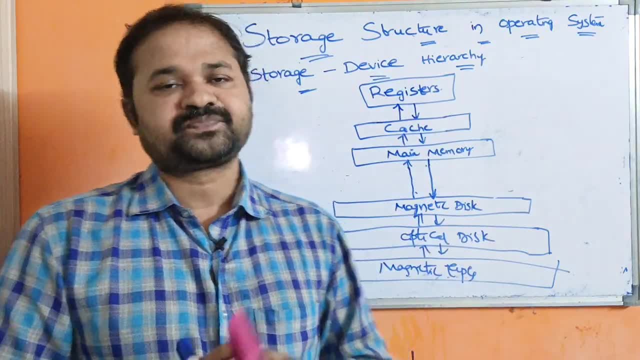 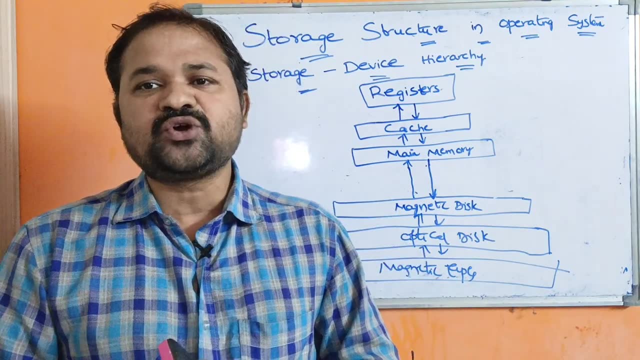 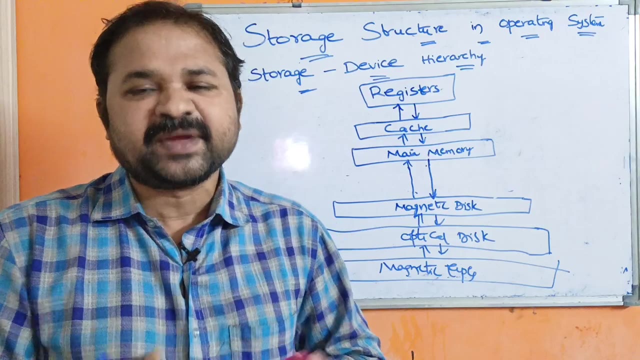 Let us see about all these devices one by one. The first one is resistors. Resistors are mainly useful in order to store a small piece of information. Resistors can store the information in the form of bits. The size of resistor may be. 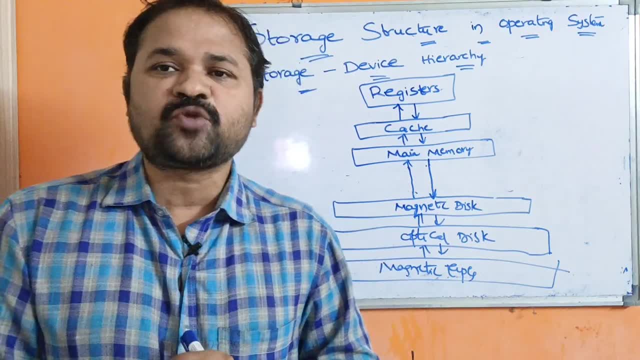 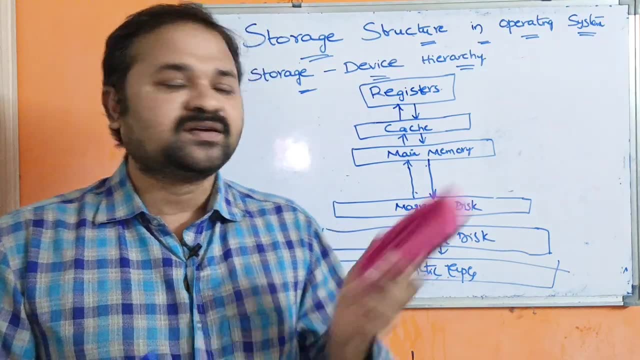 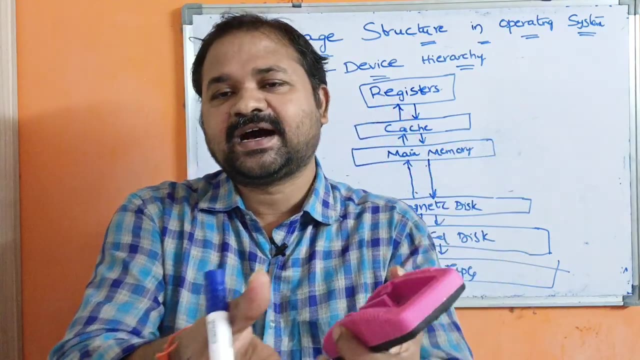 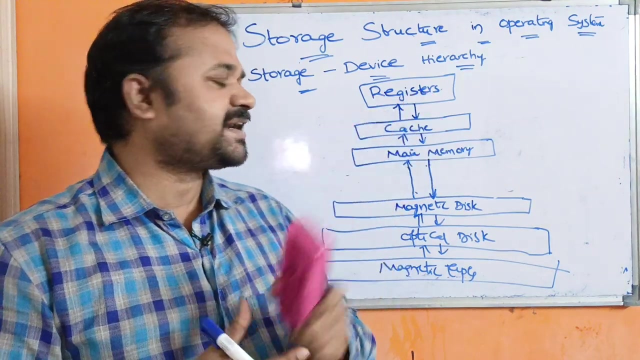 8I看一下 bits: 16 bits, 32 bits, 64 bits. likewise, the major advantage of register is cpu can access the data of registers in a faster manner. why? because registers resides very near to the cpu, so that cpu can access the data present in the registers in a faster manner. register means a collection of.